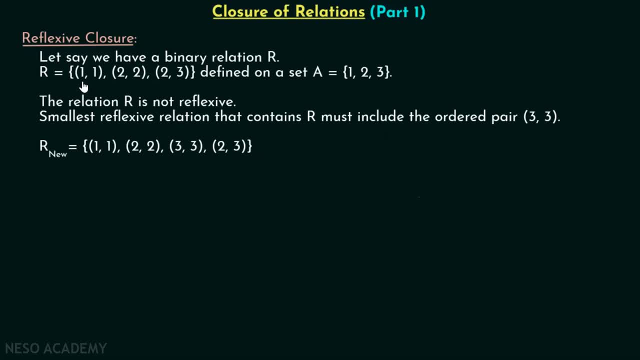 R right. So it is clear that in order to make this relation reflexive, we must include 3, 3 in this particular relation. right. Now let's come to the definition of reflexive closure. Reflexive closure of a binary relation: R on a set. A is the smallest reflexive relation of the set. A. So let's say we have a binary relation R on a set A which consists of three elements: 1, 1,, 2,, 3,, 3,, 4,, 5,, 6,, 7,, 8,, 9,, 10,, 11,, 12, and 12.. And we have to find the smallest reflexive relation. 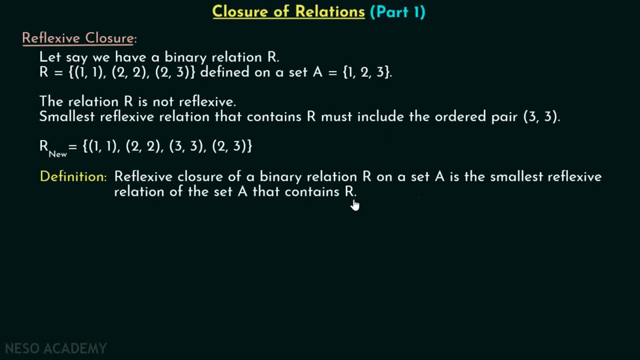 of the set A that contains R. As simple as that. So, whenever we want to find reflexive closure of a binary relation, R, we must find the smallest reflexive relation of the set A that contains R. Reflexive closure of R is usually denoted by R- R+. Okay, this is the symbol which is used to 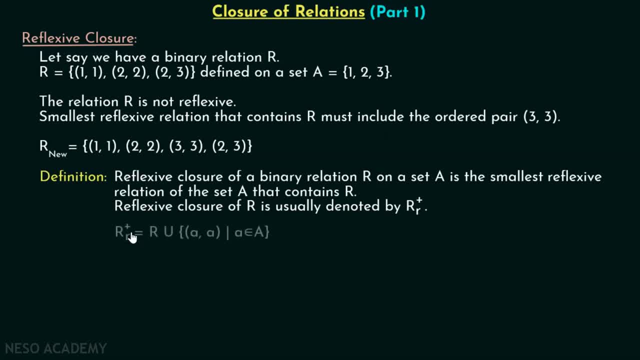 denote reflexive closure of R And formally we can say: R. R+ is equal to R. union set of all ordered pairs, A, A, such that A belongs to A. Here we are talking about some arbitrary set A. okay, Now let's discuss one problem related to reflexive closure. 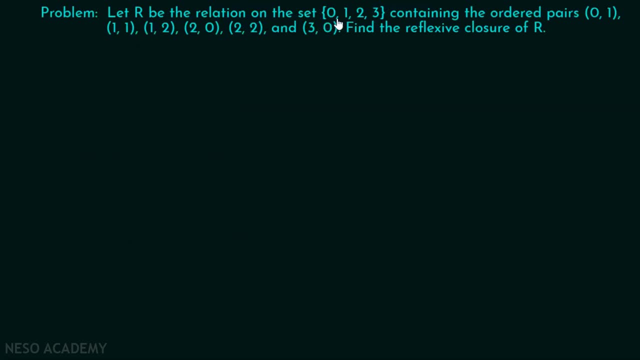 Let's discuss this problem. Let R be the relation on the set 0, 1, 2, 3, containing the ordered pairs 0, 1, 1, 1, 2, 2, 0, 2, 2 and 3, 0.. 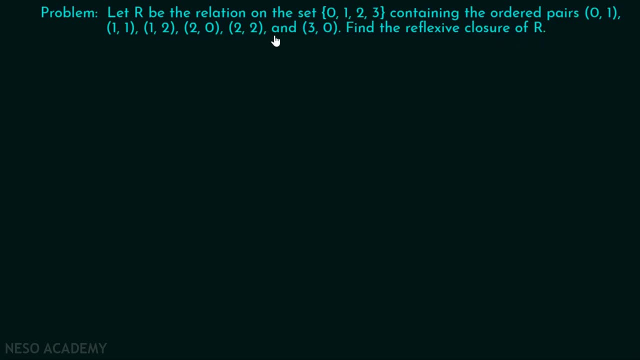 Find the reflexive closure of R. We are interested in finding the reflexive closure of this particular relation, which is defined on this set: 0,, 1,, 2, 3.. So you can think of this set as the domain of this relation. 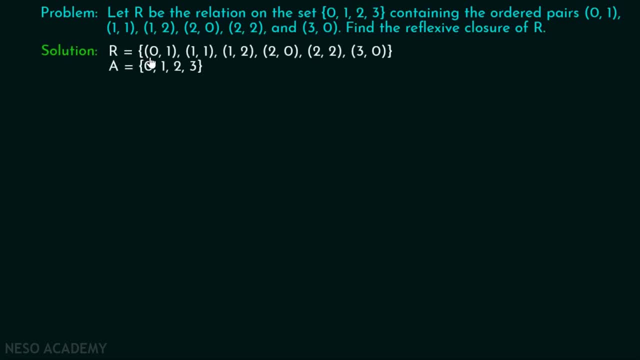 Okay, so we have a relation R which consists of these ordered pairs: 0, 1, 1, 1, 1, 2, 2, 0, 2, 2, 3, 0, and we have a set A which consists of these elements. 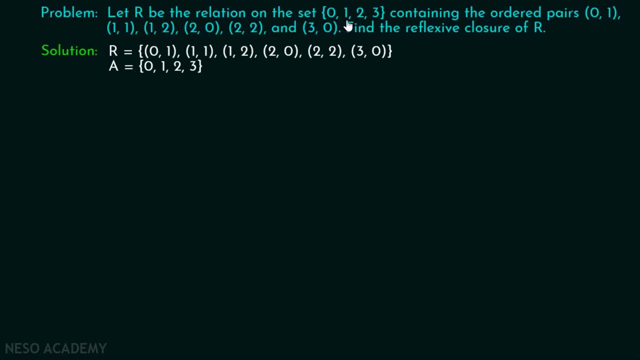 Okay, let's say this set is set A. Okay, you can choose any letter for this set doesn't matter. Okay, now we are interested in finding the reflexive closure of R. Reflexive closure of R is denoted by RR plus. 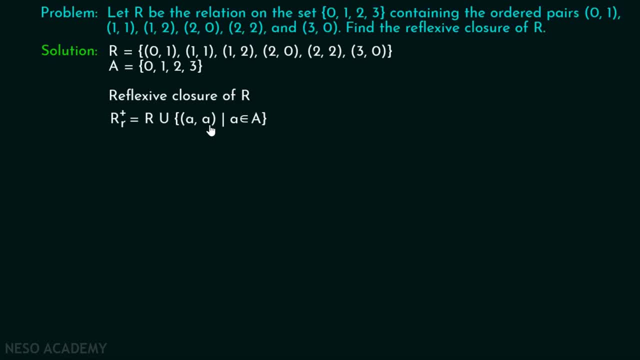 is actually equal to R union, with set of all ordered pairs A- A, such that R is the set of all ordered pairs A- A and that A belong to A. that is this particular set A. Now this means that we must include R plus.